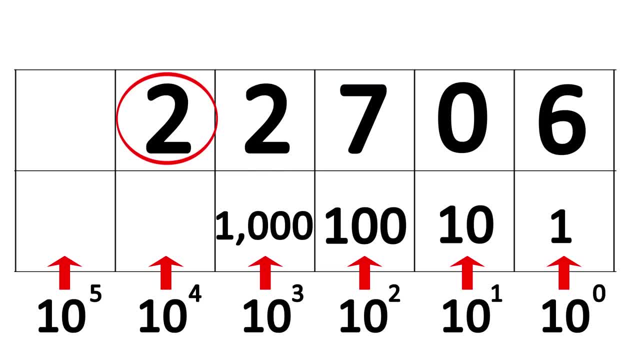 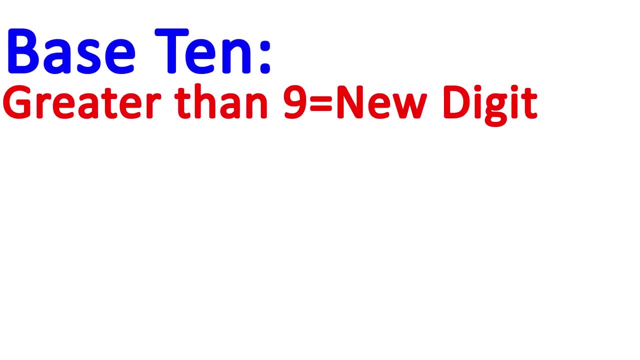 The number of tens, the number of hundreds, the number of thousands, and so on. Now, this is probably something you already know, but it's very important to keep it in mind when we talk about binary. Now, binary works the exact same way as base-10 positional. 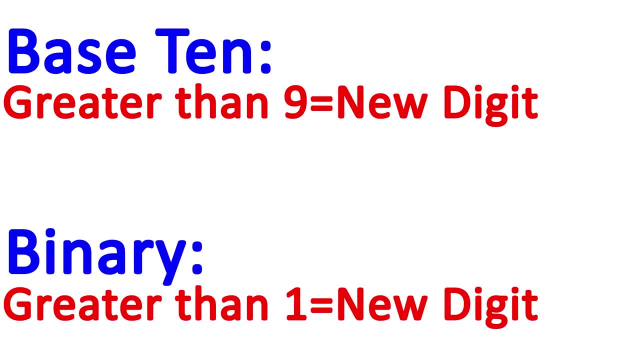 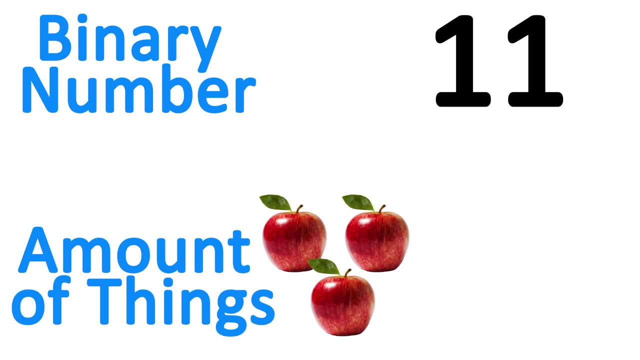 but instead of each digit going from zero to nine, it goes from zero to one. Counting upwards in binary sounds like this: Zero, one, ten, eleven, one hundred one hundred one, one hundred ten, one hundred eleven and one thousand. 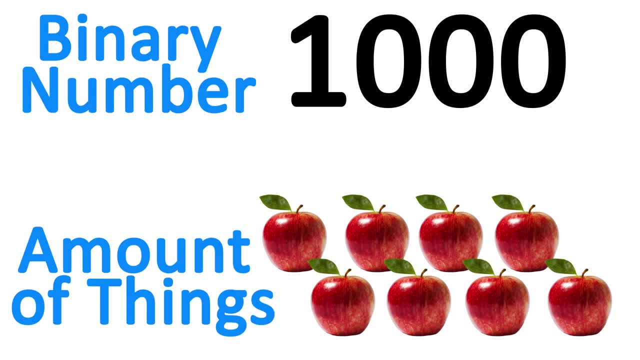 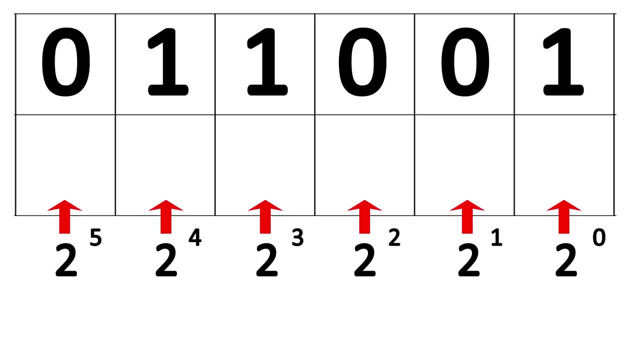 Because each digit of binary has only two values and not ten. each additional digit represents an increasing power of two rather than an increasing power of ten. So this is the number of ones we have: the number of twos, fours, eights, sixteens, thirty-twos. 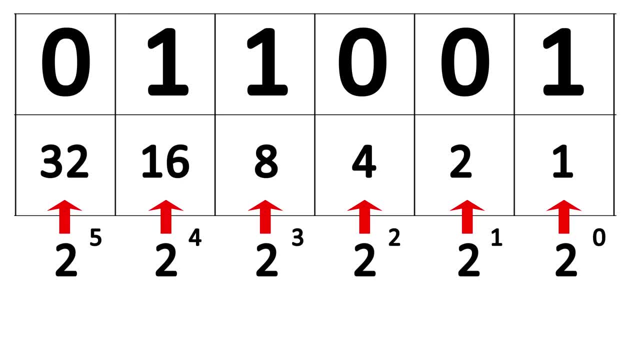 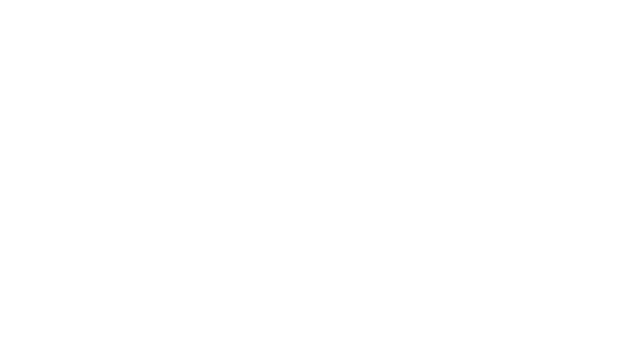 sixty-fours, one hundred twenty-eighths and so on. Not nearly as efficient as base-10, but exponentially more efficient than tally marks, Literally. So now that we know how binary works, let's talk about computers. Why did the first computer creators as wise and intelligent as 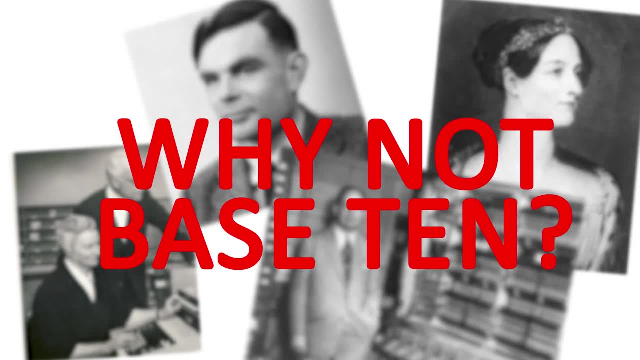 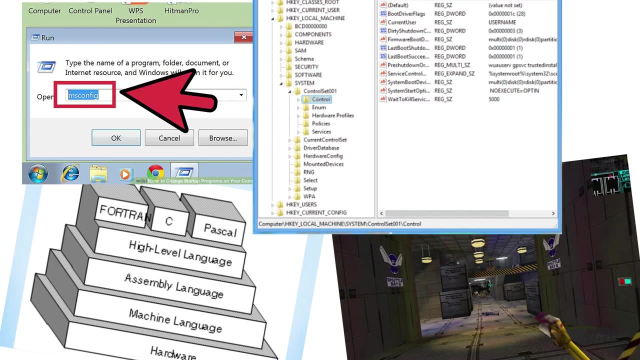 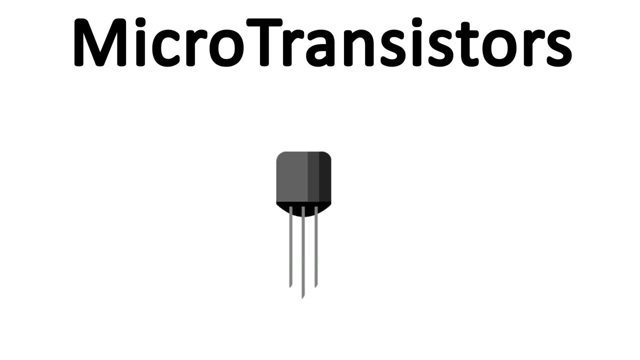 they are waste their time with such an ineffective system of counting. Well, it's because of a physical limitation on how computers work. Everything a computer does comes down to what's known as microtransistors: Simple, tiny, eensy-beensy little switches that can either be on or off, and can be flipped on. 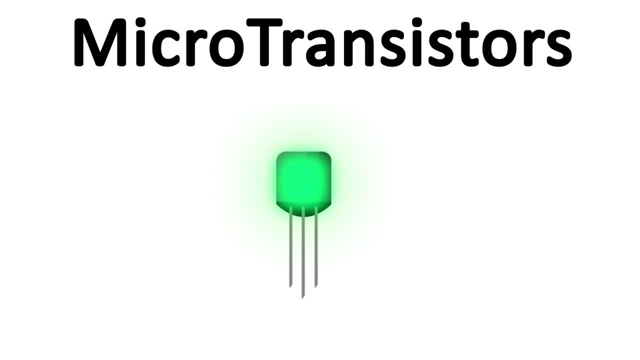 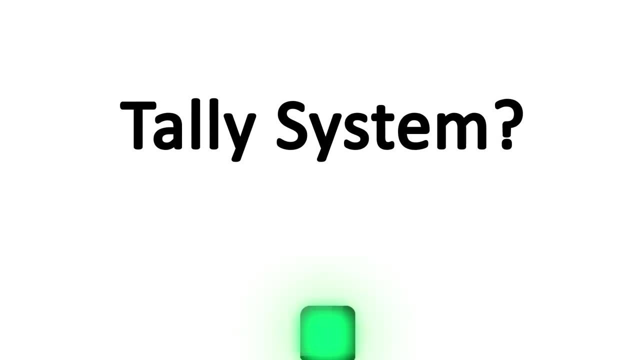 or off with a very weak electrical charge. The first goal was to get computers to count, and to get them to count by using the power of the computer. So let's talk about computers, So we can use the tally system, meaning the number of ON switches equals the number of things we have. 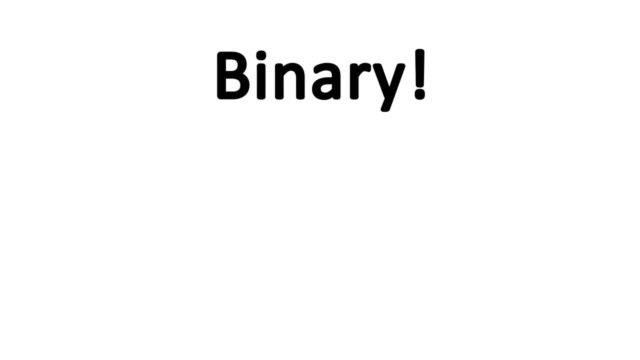 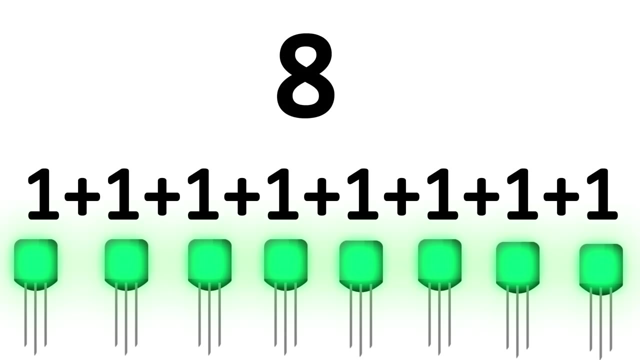 or we could use the much more efficient system of binary, where each switch represents a digit of binary. Eight transistors using the tally system could represent a number as large as eight. by turning all of them on, With binary we can represent a number as high as two hundred fifty. 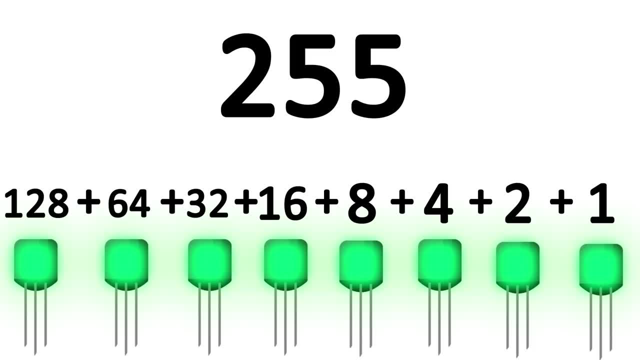 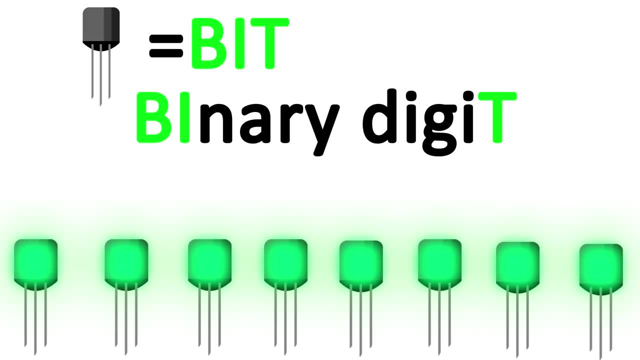 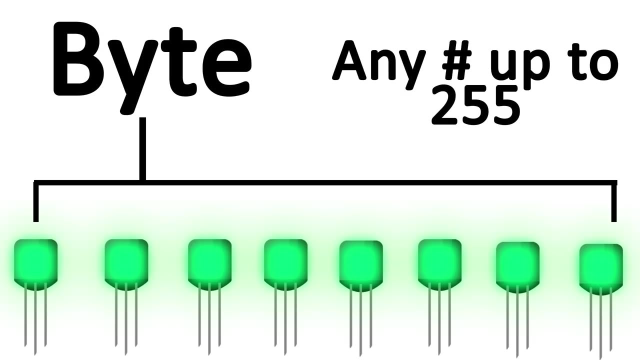 five. An ON switch means a one and an OFF switch means a zero. Now is a good time to mention that a single transistor is what's known as a bit, which stands for binary digit. A byte is eight of these bits in a row, which means any number between zero and two hundred fifty five. 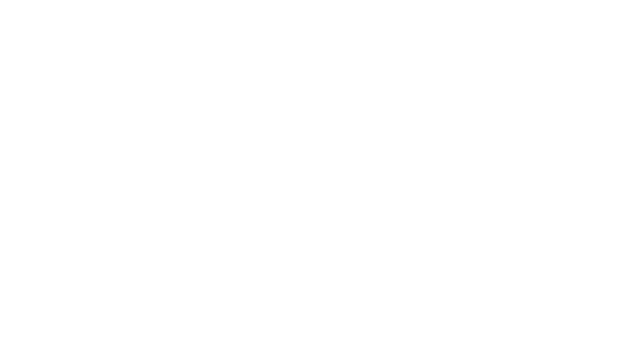 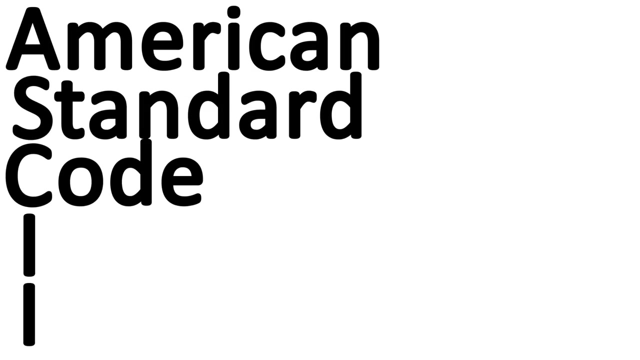 So if binary is just a system of counting, what do people mean when they explain how to spell things in binary? Well, what they really mean is how to spell things with ASCII. The American Standard Code for Information Interchange is a way to convert a computer's data. 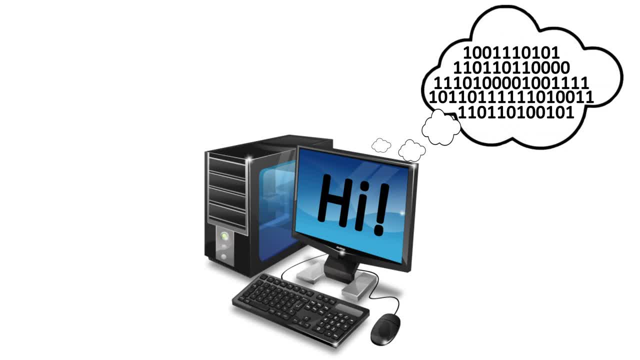 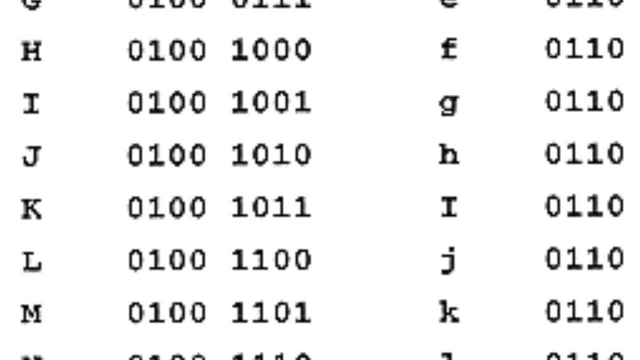 which can only be in numbers, and turn it into letters for human to have an easier time to work with. ASCII simply assigns a character to each value represented by a byte of binary And because a byte has eight digits of binary to work with and eight digits 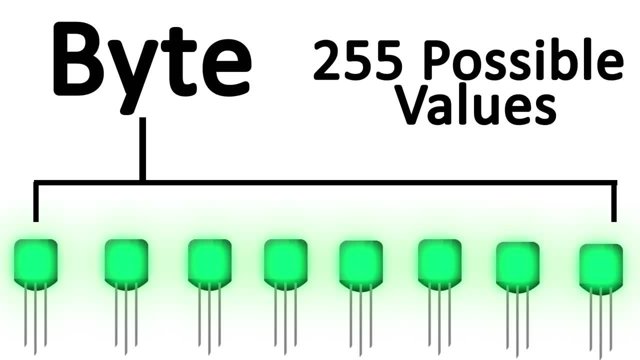 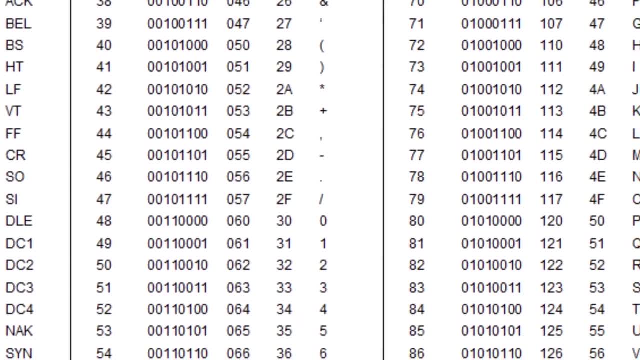 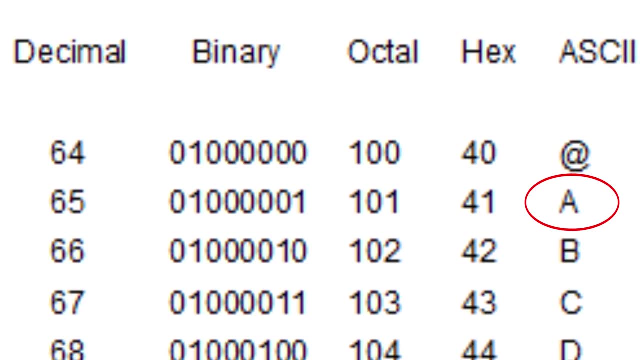 of binary can represent up to two hundred fifty five values. ASCII had two hundred fifty five letters and symbols to choose from, more than enough for the entire alphabet, punctuation marks and other symbols. For example, the corresponding ASCII number for an uppercase A is sixty five. 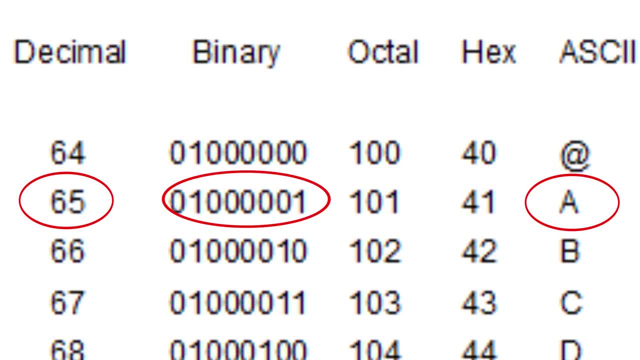 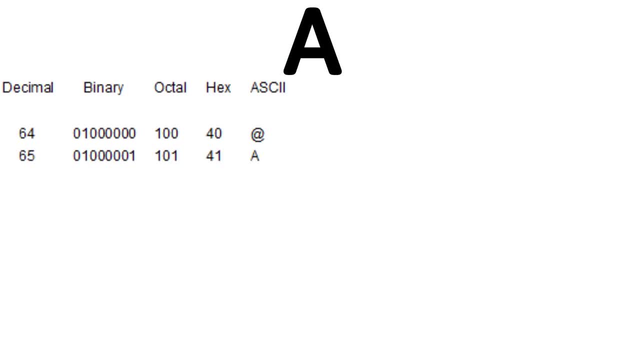 Now sixty five in base ten is equal to one million and one in binary. So whenever you type in an uppercase A in a word program, a coding program or a scripting program or whatever, somewhere there's a little tiny row of eight transistors. 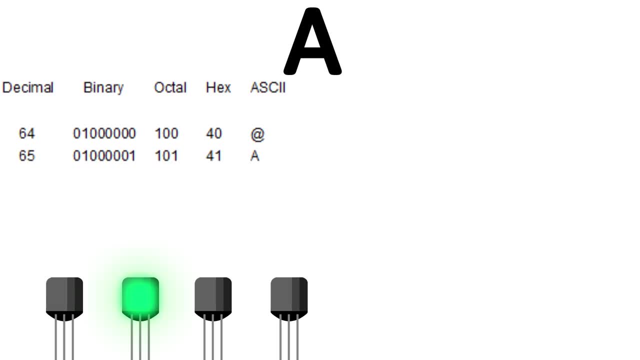 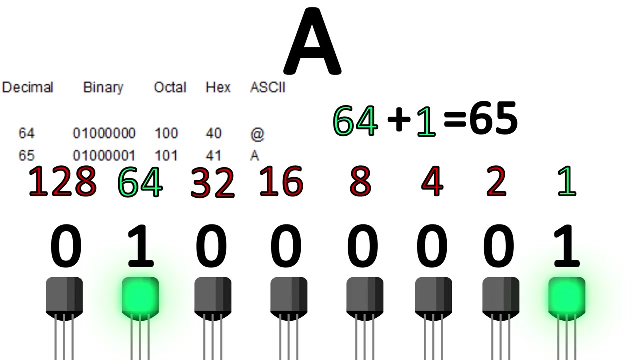 arranged in the pattern of off on, off, off, off, off off on, which represents zero one, zero, zero, zero, zero, zero, zero one, in binary, which is interpreted as sixty five, And base ten, which is converted by ASCII into an uppercase A. You're likely starting to get a feel. 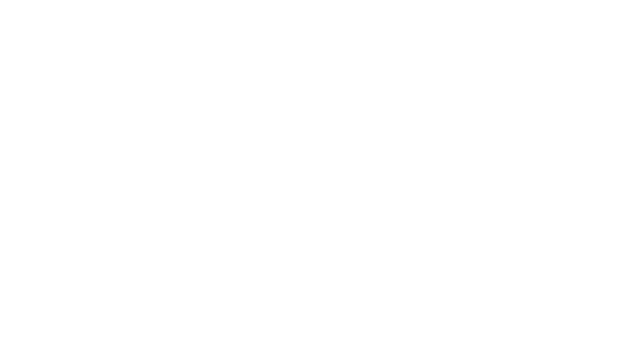 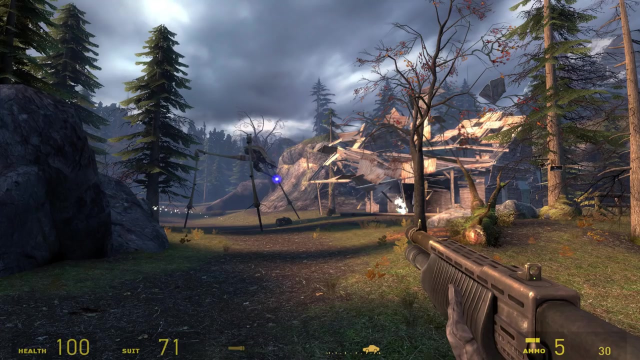 for the staggering amount of transistors required to write something as simple as a Facebook status, let alone all the different coding that your computer has to do to make the screen light up, play games, calculate massive values and so on. Well, long before we got to the point where your 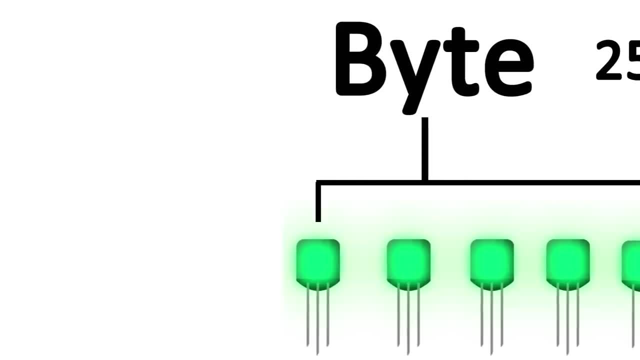 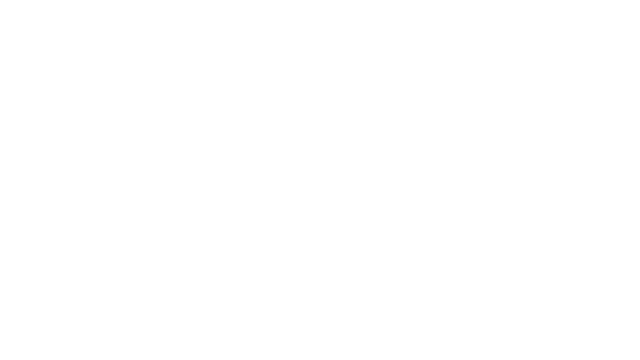 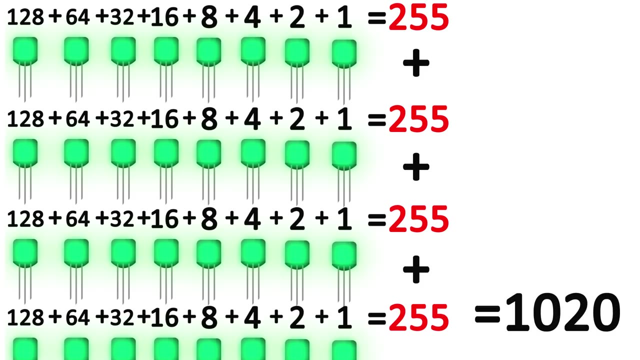 phone can play three dimensional games, it became clear that numbers as high as two hundred fifty five just weren't going to cut it, Regardless of how many bytes we had- and it was a lot. even adding four fully active bytes together could only get a number as high as one thousand twenty To solve this problem,